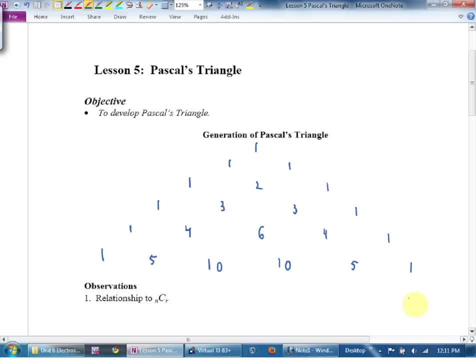 And I'll just do the first six rows, And this may not yet seem very profound, but actually it's hugely profound, okay? So I'd like you, when you do your triangle, stop at the one. five, ten, ten, five, one row. What row number is? 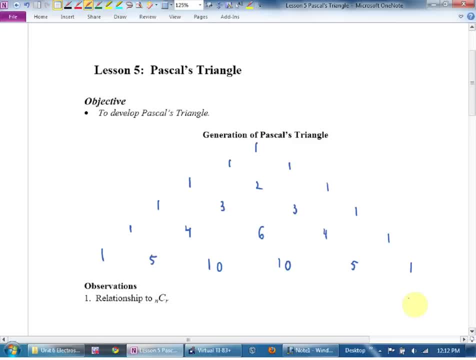 that Count carefully, Row number six And row number six is going to be the generation of Pascal's triangle. Row number six: what's the second number of row number six? Five. Row number five: what's the second number of row? number five, Four. In other words, there is a way to glance at this. 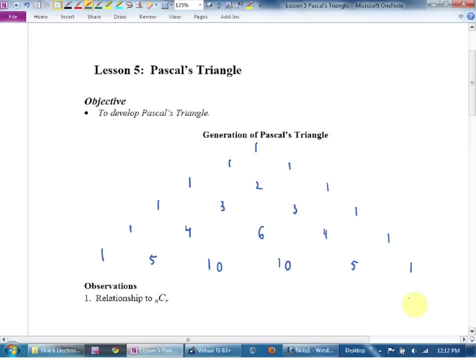 and tell what row you're in. You have to add one to the second number if you don't feel like counting over the top. I'm actually going to make a little note here in a different color, I'm going to put a little arrow here and I'm going to say: this is row six. What are some of the patterns? 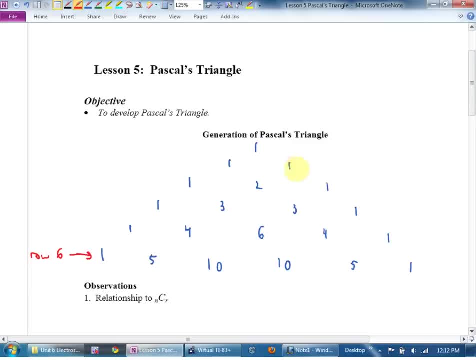 that people have spotted. Well, the first one is fairly easy. I'm going to put a little arrow here, because it's pretty obvious. If you go down this row, or you go down this row, what's the next number down here? Six, then. Okay, that's a pretty obvious one. Anybody see any other ones? 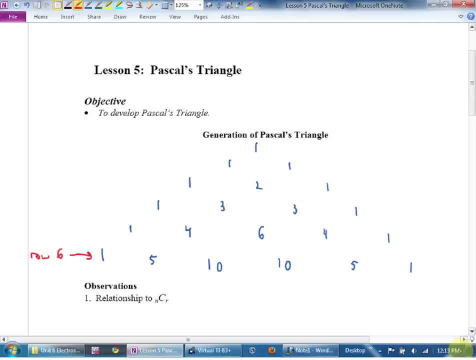 By the way, it's called Pascal's triangle because Blaise Pascal, a mathematician, wrote a book on it, but he did not discover it. In fact, there is an ancient two and a half thousand- sorry, two and a half, yeah, two and a half thousand- year old inscription, I think. 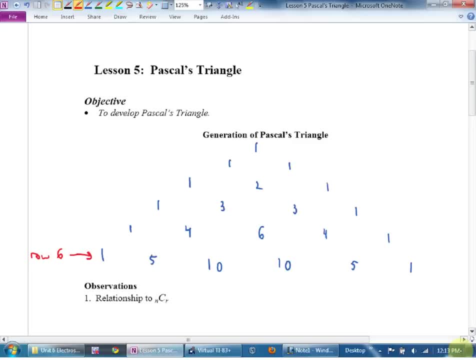 from China and it has Pascal's triangle on it. People have been fascinated by this. First of all, it's easy to draw Megan. it's kind of nerdily fun to draw. We get to add and make a triangle, but there's all sorts of patterns. 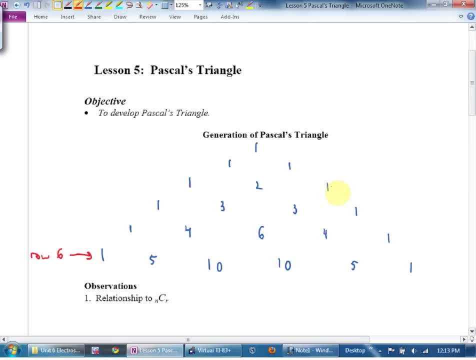 Let me show you one. What do you see? What's one plus two. Oh sorry, where are you seeing? one plus two plus three plus four? Which row, Which diagonal, Third diagonal, This one here? What's one plus three? 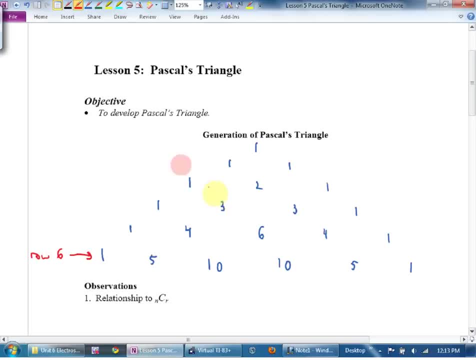 What's one plus three? What's one plus sorry? what's three plus six? Nine? What's six plus ten? Sixteen? Did you just say four, nine and sixteen? I've heard the numbers four, nine and sixteen on a list before. 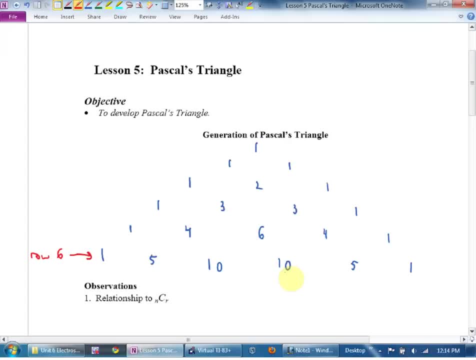 What numbers do four, nine and sixteen belong to? Really? What numbers do four, nine and sixteen belong to boy? Is it girls Tally, Not square roots? I've got to be fussy The other way. 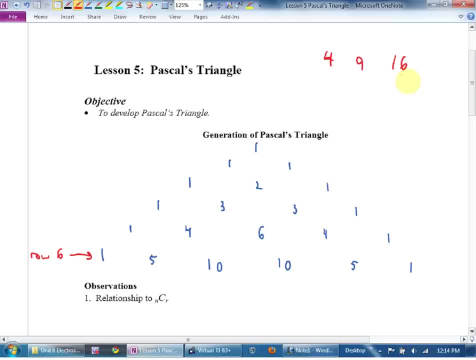 Perfect squares, The perfect squares, In other words, the perfect squares are hidden in here Further down. perfect cubes show up as well. All sorts of weird stuff starts to show up, But what does that have to do with us? What row number? 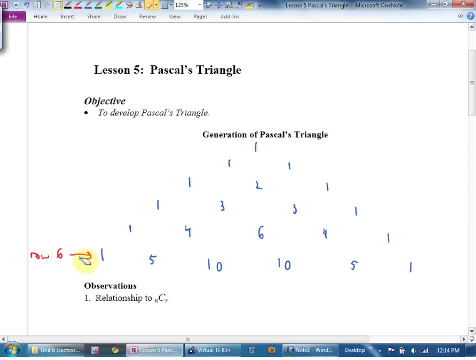 Can you, on your calculator, go: six choose zero? All of you, Yes, but we're gonna do a bunch more. By the way, I, like Kim said, isn't it just one? Yes, Six choose zero is one. Okay, What's six choose one? 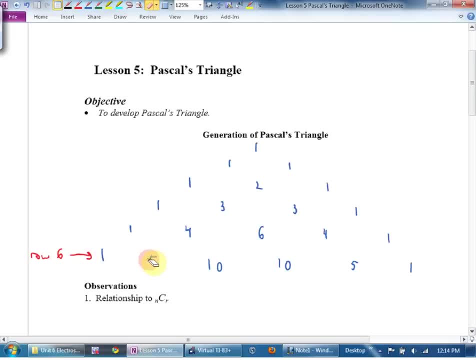 Oh, hmm, You know what, Instead of six, let's try five, choose one. What's five, choose two. Try it Ten. really No, What's five, choose three. Is it also ten? What's five, choose four. 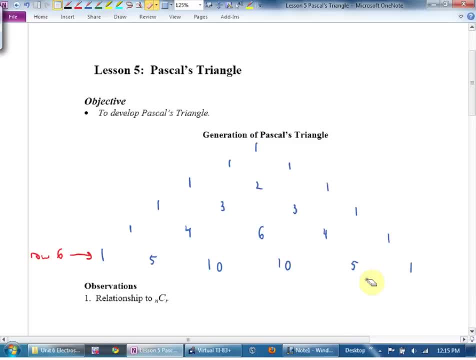 What's five choose five? In fact, row six has the five chooses. Here's how I remember that It has the five chooses and the reason. by the way, how many numbers are there in this row? The reason for five chooses: you need six items. 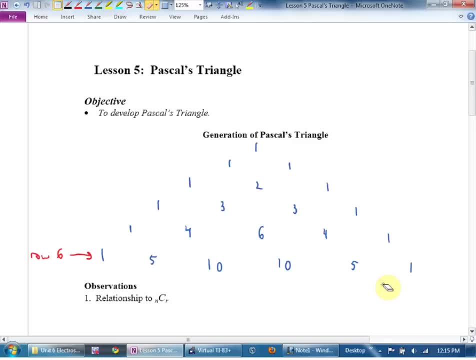 is we have to include zero as a choice. Okay, This here is actually: four choose zero. four choose one. four choose two. four choose three. four choose four. If you ever wondered, hey, how did they do this a hundred years ago? 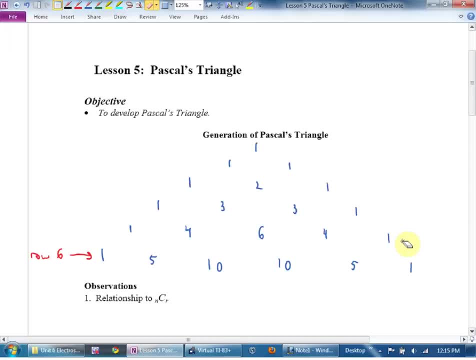 with no calculators. They had in the back of their book trig tables- Remember we talked about that for trig- But they would have had a great big Pascal's triangle, probably going up to about row twenty, And they would have limited their questions to twenty objects or less. But 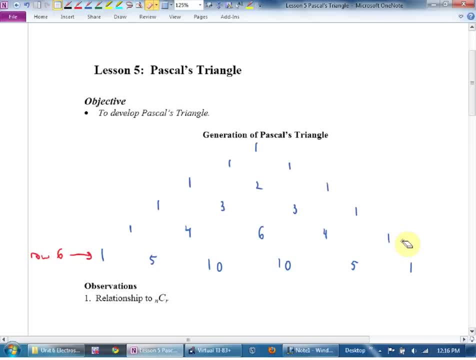 you would have had all the chooses there, Or really in a pinch, in fifteen minutes. you could generate it all yourself by doing some fairly simple in your head addition. This is: this is not counting. This is zero. choose zero One. choose zero one. 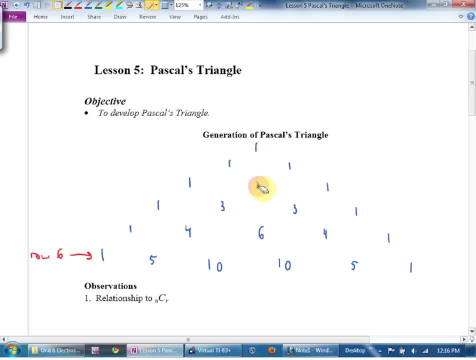 choose one. Two, choose zero. two. choose one. two, choose two. Three, choose zero. three choose one. three. choose two. three choose three. See it Now. we're going to try and write that algebraically, So are you ready? 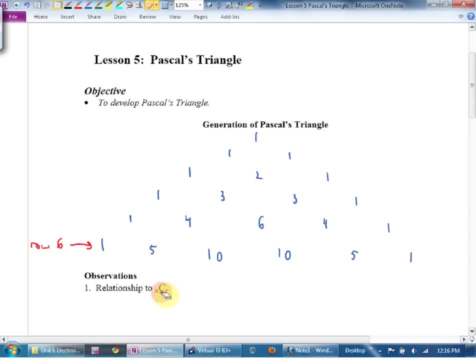 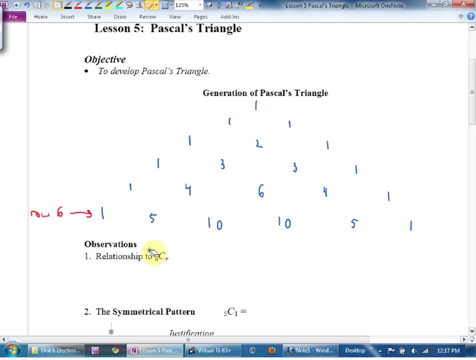 What's the relationship to n choose r? If we're in row six, this is the five here. how does that work? What's the relationship to n choose r? I'm going to call this row six and I'm going to call this term one. 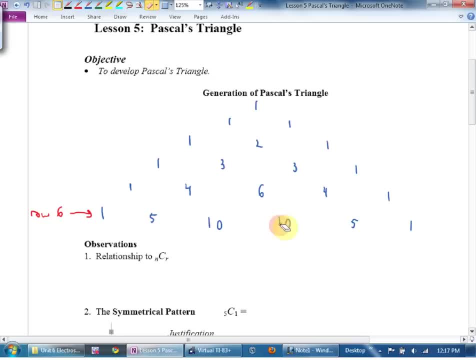 term two, term three, term four, et cetera. So if I want to find the fifth term in row twelve, The fifth term in the twelfth row, Now look up for a second. Here is the first term in the sixth row. What is? 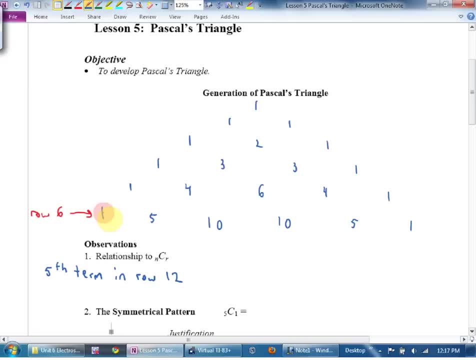 that What, choose what? So I'm just going to write this down. You don't need to write this down, But you said first term sixth row was five: choose zero. Is that right? What would the third term in the sixth row be? 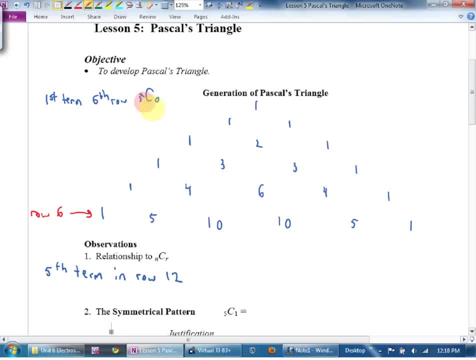 Five, choose two. So can you spot the pattern? If I want the twelfth row and the fifth term, it's going to be eleven. choose four, One less, one less And on your test, Vitaly as a multiple choice question. 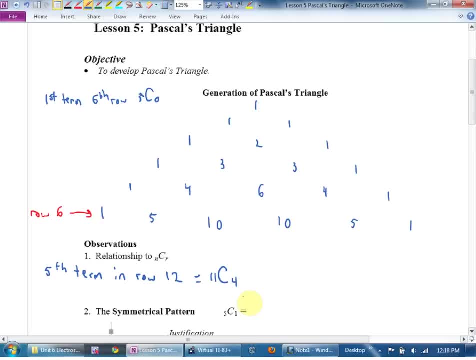 I'm going to say to you: tell me the sixteenth term in the nineteenth row of Pascal's triangle, By the way. what is the fifth term of the twelfth row? What is it? Sorry, 330?? What is the eighteenth term? 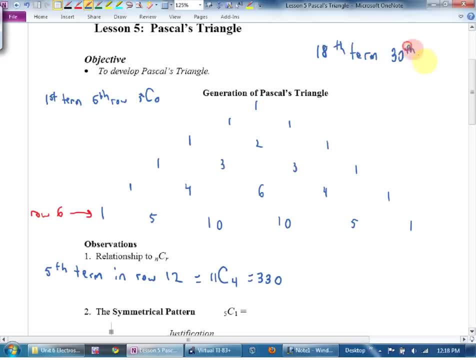 of the thirtieth row: What choose? what Twenty-nine choose seventeen. Now I do say: memorize that, Although if you blank out, you can draw this and figure it out, But it would take you about two or three minutes to derive it. 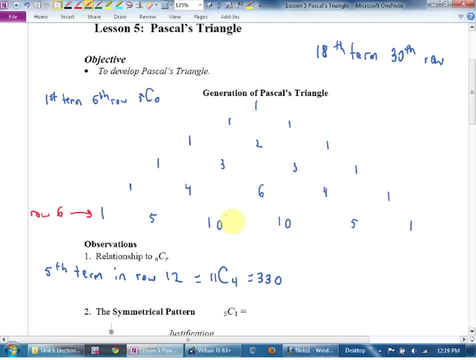 It's worth memorizing. One less, one less. By the way, what is twenty-nine? choose seventeen, So they do get fairly big eventually. It's funny: when I first did this about eight years ago, I asked for the twelfth term of the fourteenth. 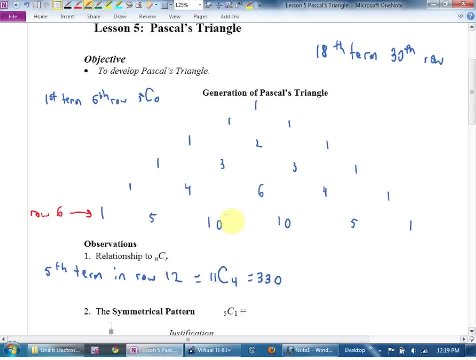 row and I still had about half my kids write out the whole triangle. So the next year I said: okay, instead of the fourteenth row I'll make it the eighteenth row, And I still had about ten of my kids write out. 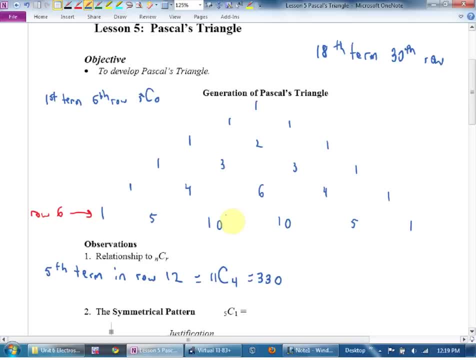 Pascal's triangle. So the question has slowly gotten bigger and bigger and bigger every couple of years. I'm like I want them to use the shortcut. I don't want to see a back page full of an entire triangle or a piece of scrap paper stapled to it. 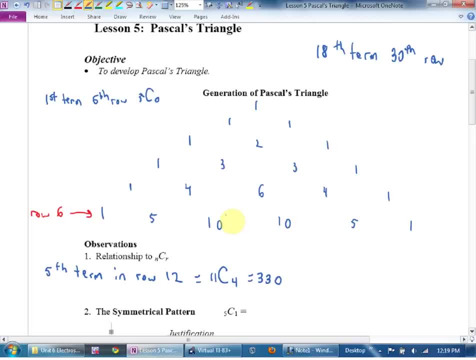 where someone's written out eighteen rows of Pascal's triangle. We're trying to find shortcuts, We're trying to count without counting, Right. Okay, Then there is a symmetrical pattern. Here is: five, choose one. What's this? Five, choose. 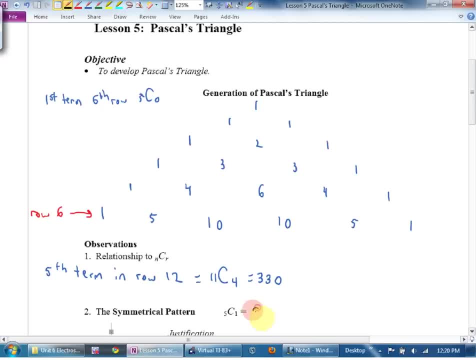 Five choose one is the same as five choose four, And we talked about why the other day. We said: look, if you're starting with five people, if you're forming groups of one, you're automatically forming groups of four, because that's who's left behind. 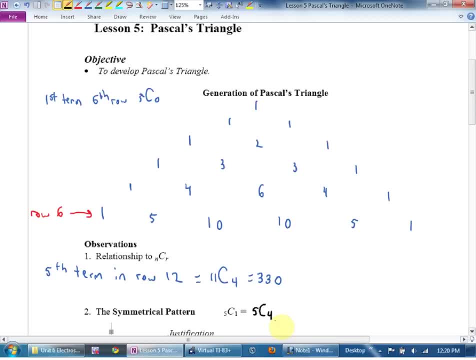 And you'll have the same number of groups, whether you go one person and leave four behind, or four people leave one behind. You can't form a group of one without forming a group of four. You can't form a group of three without automatically forming a group of. 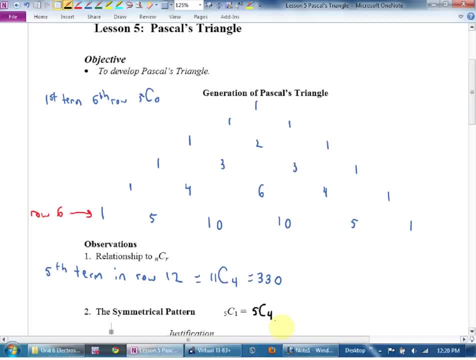 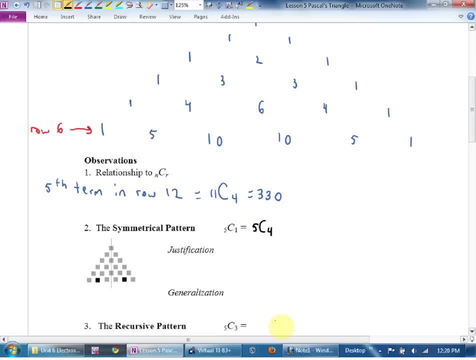 two. if we're talking about five people, Okay, If we want to generalize that, we would say this: n choose r equals n choose. Can you look at this and write this algebraically? but instead of a one, put an r there. 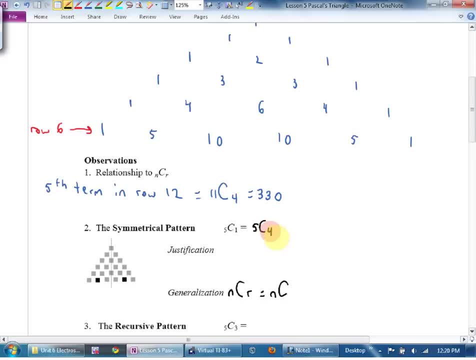 Instead of a four. what would you put there? How did we get the four based on n minus r? As it turns out for what it's worth algebraically, n choose r is the same as n choose r, n minus r. 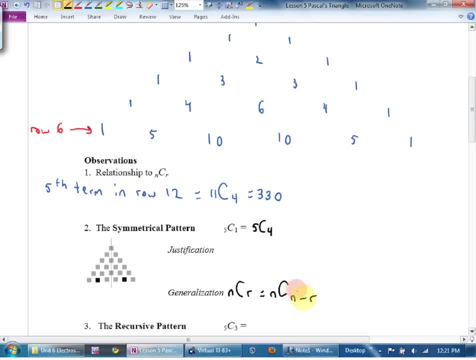 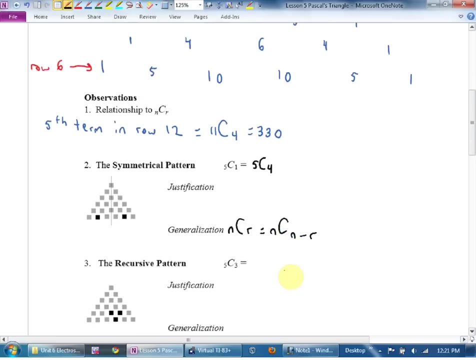 I don't memorize that, I know this And I think you guys picked up on that last class. There is also a recursive pattern. Look up, I'm going to erase some of this triangle and I'm going to write it in terms of choose. So what's this? 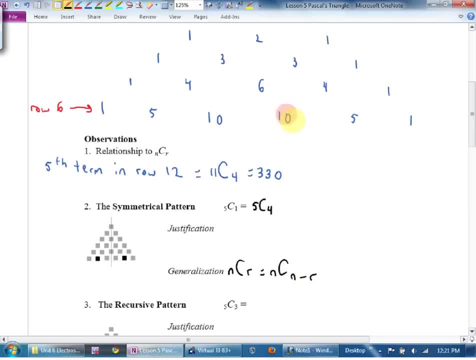 in terms of: choose Five, choose what Five choose zero five. choose one, five choose two. What's this guy? I'm going to erase this and put a five choose three there. You guys don't need to, I just want to spot the pattern. 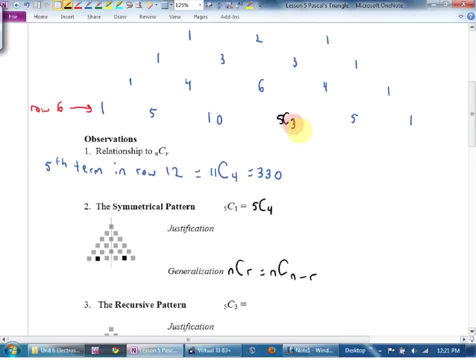 But where did this ten come from? It came from those two added: Oh, what is this in terms of a choose? I'll give you a hint. Four, choose what? Choose zero, choose one. Oh, this is four. choose two, And what's this one? 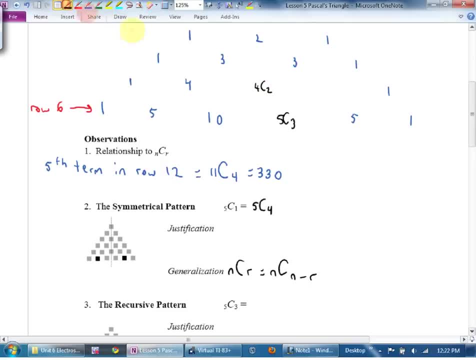 here. So, as it turns out in terms of a recursive pattern, four choose two plus four choose three, equals five choose three Or five, go bigger numbers, Mr Dewitt. So spot this, See if you can spot this next one then. 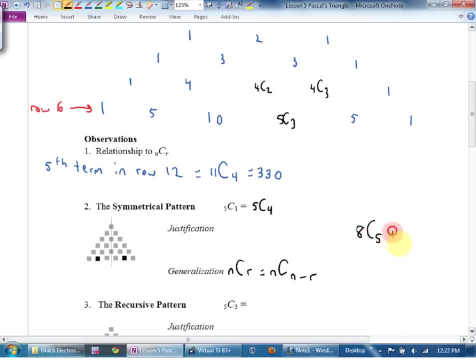 Eight choose five plus eight choose six would be equal to nine choose six. See it Big deal. Well, Matt. what this is saying is: don't forget how Pascal's triangle is generated. There is a recursive pattern. The next term came from the two above it. 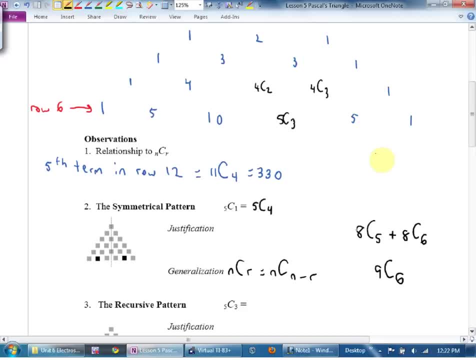 The next term came from the two above it. I'll be completely honest: I don't memorize the choose part at all And in fact, I'm going to do something different this year. I'm not even going to write the choose part here. 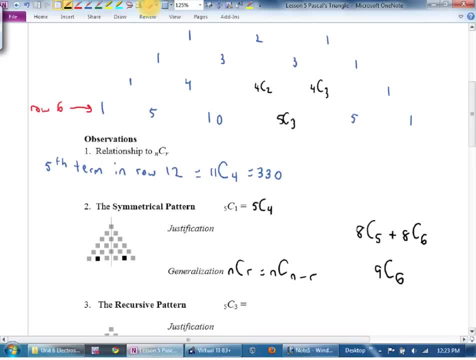 What you do need to know for Pascal's triangle is not the chooses that. this choose this plus this choose this equals this choose this. What you do need to know for Pascal's triangle is that six and four gave you a ten. You need to know how to generate it numerically. 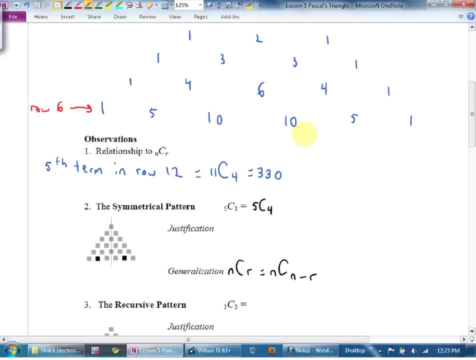 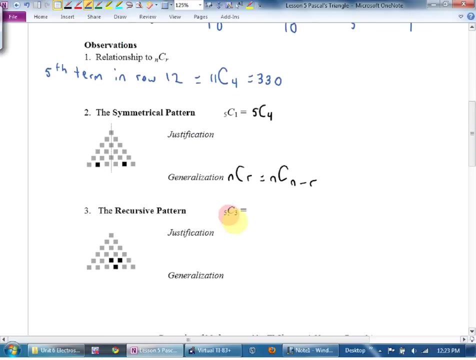 not algebraically. Do you understand the difference in vocabulary? No, you were late. Don't think about running water or water balloon versing or anything like that. So for the recursive pattern, for what it's worth, this would be four. choose two plus. 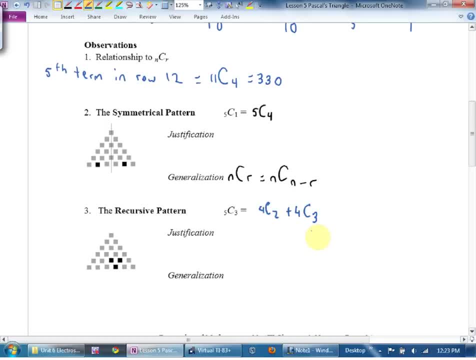 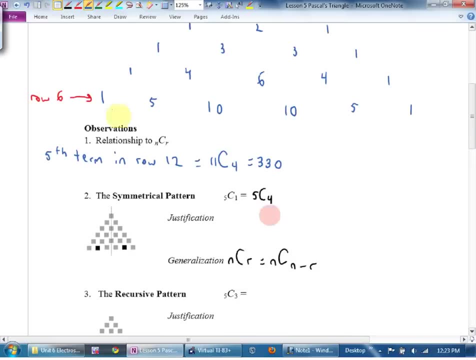 four, choose three, But you know what? Don't write it down, Cross it out. You don't need to know that. You need to know, though, that like: could you all find the next row for me? Yes, In fact. 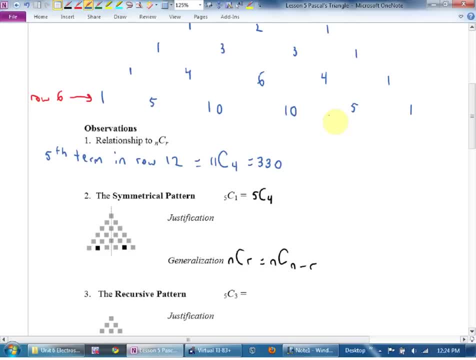 what Pascal's triangle questions am I going to ask you on the test? I am definitely going to ask you that one. there Find me the twelfth term of the nineteenth row. It'll be a multiple choice, Oh, and I'll even tell you what the 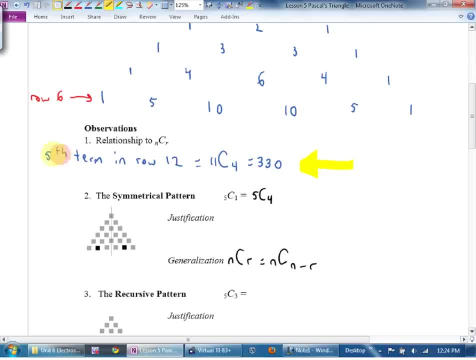 answers will well for this question here. I'll even tell you what I'll use for my answers. One of the answers will be twelve: choose five. One will be twelve: choose four. One will be eleven: choose five. One will be eleven. choose four- The correct one. 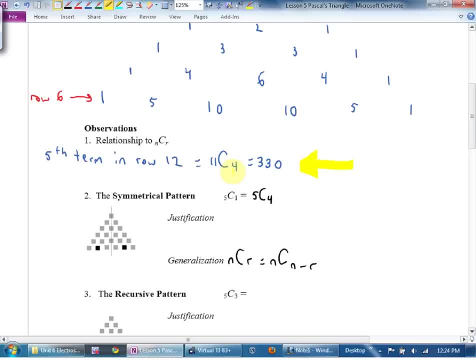 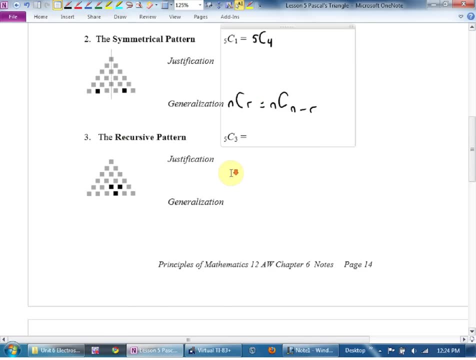 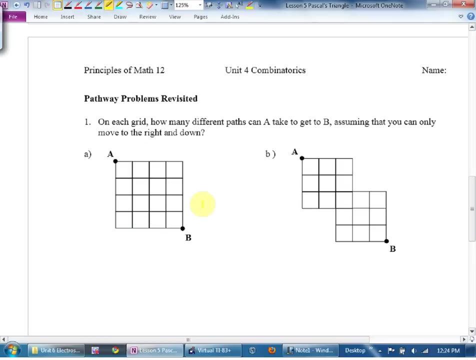 There's an even nerdier, cooler use for Pascal's triangle and it comes up in irregular pathway problems. Next page over Here I have for you two pathway problems. We call this one a regular pathway. We call this one an irregular pathway. It's difficult. 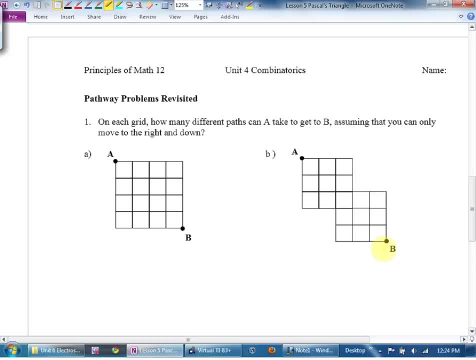 for me in English to explain what makes an irregular pathway. but can you see with this diagram what I mean by an irregular pathway? There's overlapping. Okay, Yeah, Okay, Okay, If we want to solve this. how many pathways if we're always moving right and down? 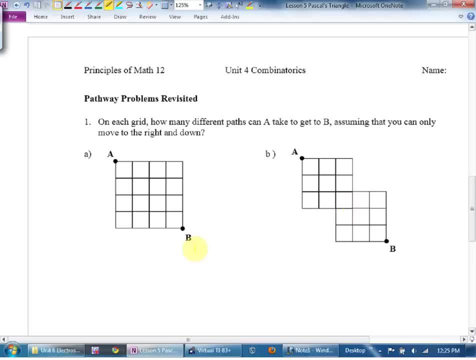 Now the method that I gave you initially: don't write this down for a regular pathway problem. don't write this down. was this Right, right, right, right, down, down, down down? and we said: that was what factorial. 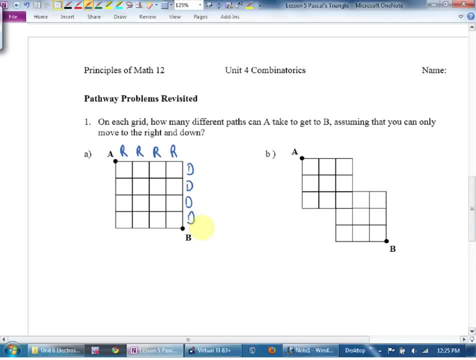 over what factorial? what factorial? No, How many letters in this word. Eight factorial over four. factorial, four factorial. Now, by the way, by a nice coincidence, that happens to be eight. choose four, which is faster to type than eight. factorial over four factorial. 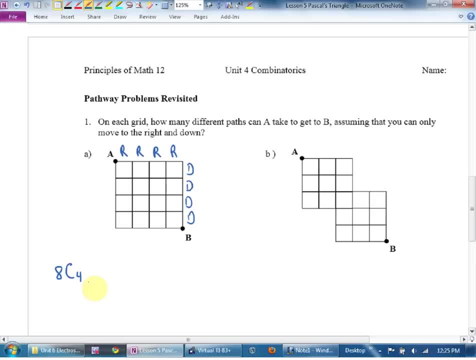 four factorial. So if this was a two by four rectangle, it would be six choose two, or six choose four. You get the same answer, no matter what. That method does not work here, By the way. what is the answer? What is? 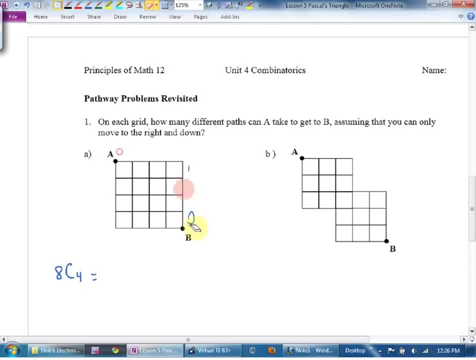 eight choose four. or what is eight factorial over four factorial, four factorial. What do you get? Seventy. Write that down. So I'd like you to write down here: eight choose four, seventy. The problem is the factorial shortcut. 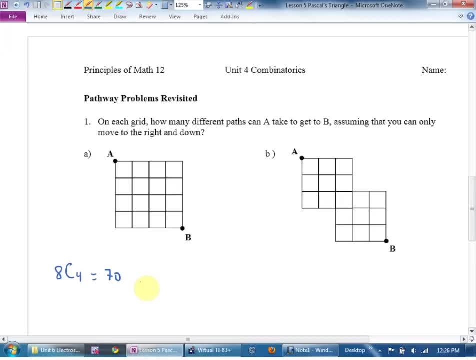 only works for regular pathways, Not for irregular ones. So I want to show you a different way to get the answer, and somewhere along the way, maybe you might even all of you- start to smile with your inner nerd, Because it's grade three math. 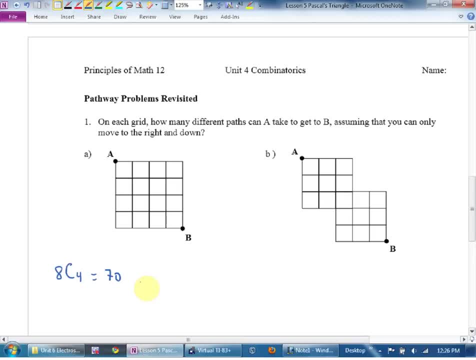 to solve a grade twelve question. But to do that I need you to put your pencils down, And what I would like you guys to do is rotate your page forty-five degrees so that A is vertically right above the B. Spin your page. I can't do. 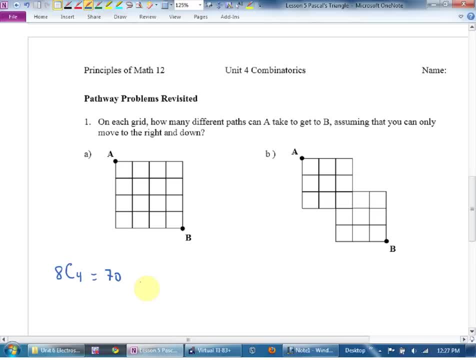 it up here but spin like so, that, like that, So that the A is right above the B. Spin it like that Boy. that was a dumb movement to do it. Good enough, Okay, Y'all done that. 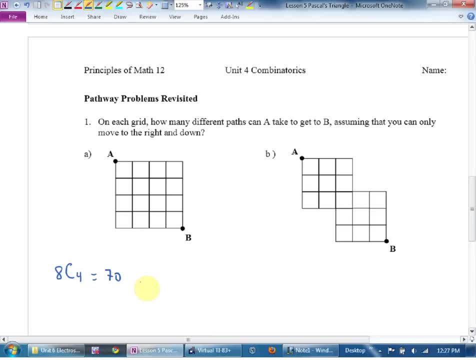 Rio, no, you haven't spun it yet. Spin it, Tilt your paper. Yeah, So the A is right above the B. I'm serious, All of you I'm serious And then watch. So I can't do this, I gotta. 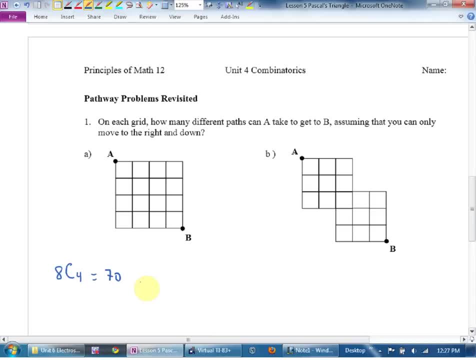 turn my head and it makes it way way tougher. But watch, I'm gonna put a one there. I'm gonna put a one there and a one there. I'm gonna put a one there. You know what I'm gonna put right here. 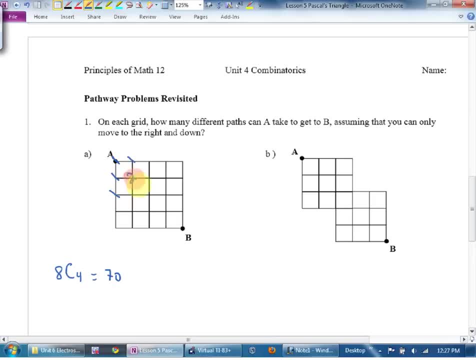 Two, A one there. I'm gonna put a one there. You know what I'm gonna put right here: Three, Three, One, One. What's gonna go here? Four, Six, Four, One. Let me zoom in. 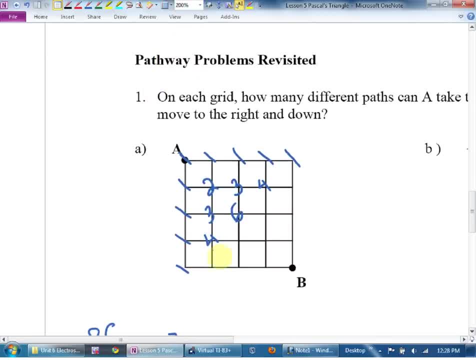 What's gonna go right here? What's gonna? Don't write this down yet. Watch, Put your pencils down, Cause you're gonna do this yourself afterwards for practice. What's gonna go right here? Five: What about here? What about here? 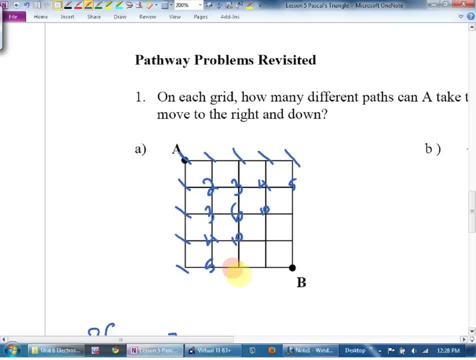 What about here, Here, Here, Here Here, Pascal's triangle? Now, I would never do a regular one this way, but the nice thing is this will work for the weird one next to it when the factorials won't, So try. 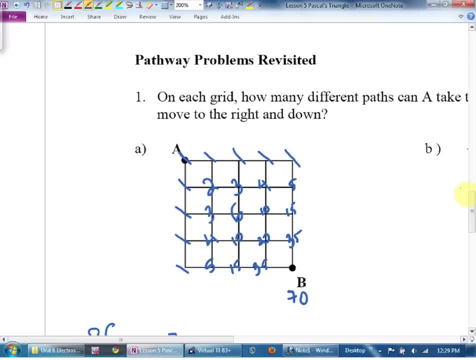 this on your own now. And, by the way, do you see why I said tilt the paper? It's way easier to work straight down. Trust me, Trust me, Try filling this in on your own without copying mine out, And then. 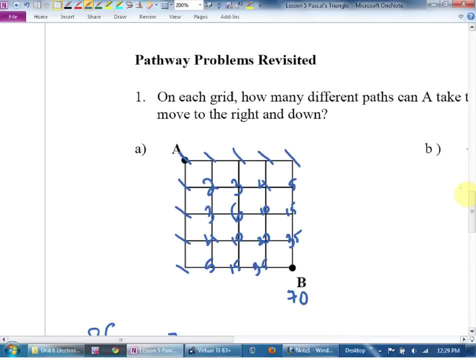 I'm gonna try the great big one and then I'm gonna pull it off the screen and let you try the great big one on your own. That means my little corner of three ladies over there when I do the great big one. 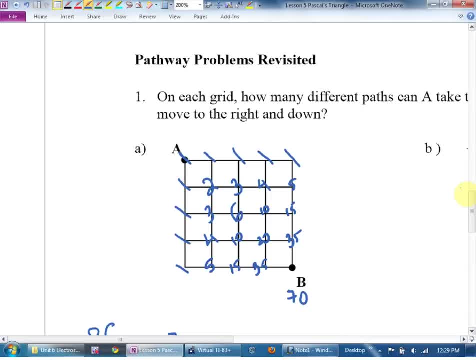 you're not gonna write anything down while I'm doing it. Then you'll try recreating it afterwards. Come on, that is nerdily cool, though that it works. Now, Jasmine, I'm not gonna prove to you that it works for the irregular ones. 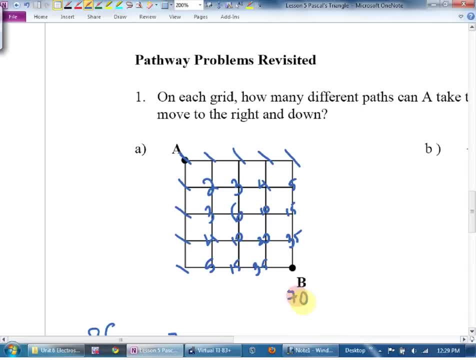 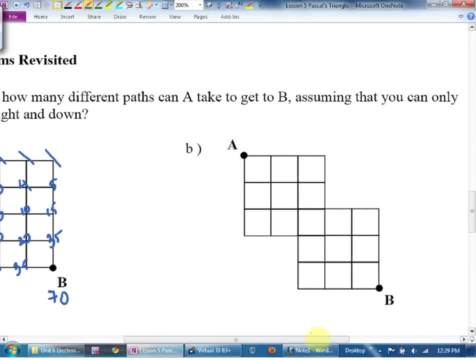 but we're just gonna say: it worked for this, it will work for this as well. I really wish I could rotate this about 45 degrees. Sadly I can't. Uh, except this is the way I've done this. I've done it as a 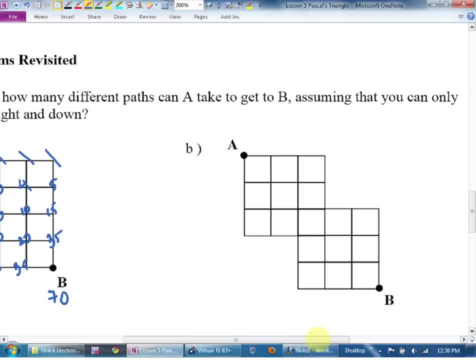 JPEG. so no, In my Word original file yes, and that's what I used to do, But I'm not desperate enough to try and fix that right now. Let's try the next one. Look up, Watch Ready. Don't write this down, just watch and see if. 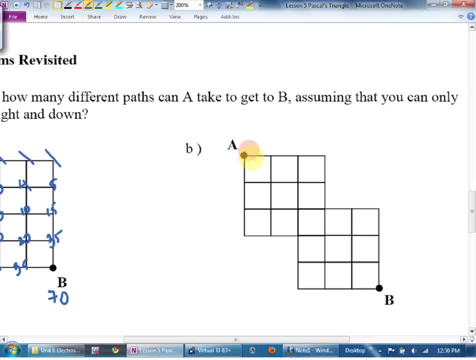 you can derive this with me: One. What's gonna go here? Yeah, by the way, what I'm really doing is saying, oh, and right here there's an invisible number, right there, What Zero? I'm going zero plus one, so one. 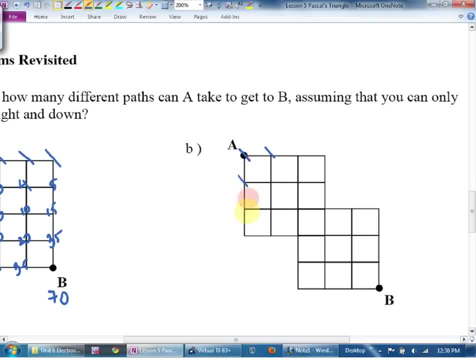 one, one, two, one, and always go one complete row at a time. Don't try and work your head down one side. you'll screw up. What's gonna go here, Here, Here, Here, It's gonna go here. 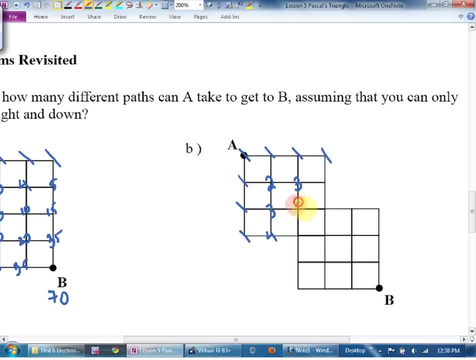 Four: What's gonna go here? What number's right here? It's invisible. Zero and a ten: What number's gonna go here? The ten just slides down. Twenty, Ten plus zero, ten, Ten plus zero, ten Thirty. 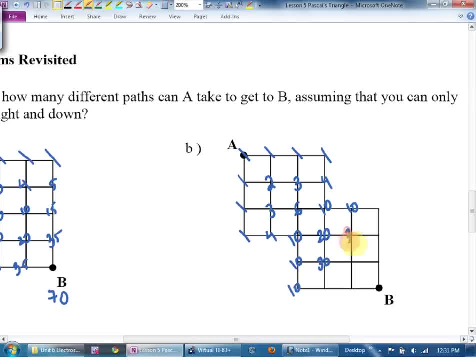 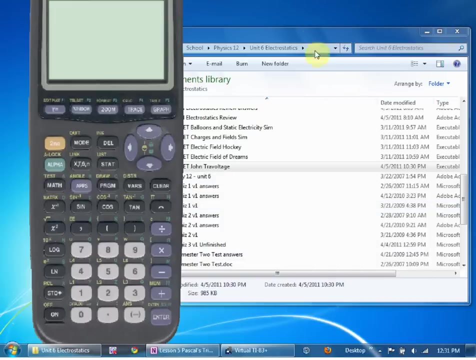 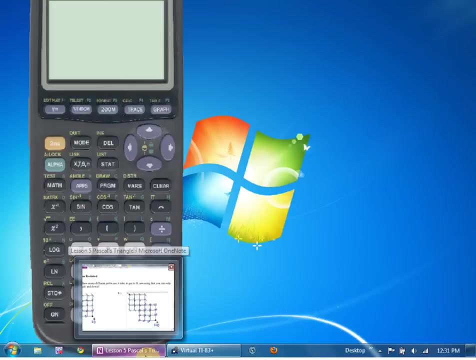 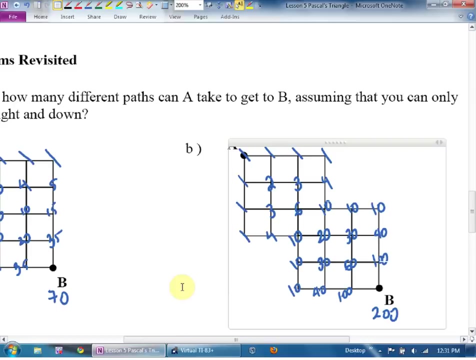 Thirty, Ten, Forty, Sixty, Forty, One hundred One hundred Two hundred. Try it On your own. Three, One hundred One hundred Two. One hundred Sixty One hundred, Three, Three, Four. 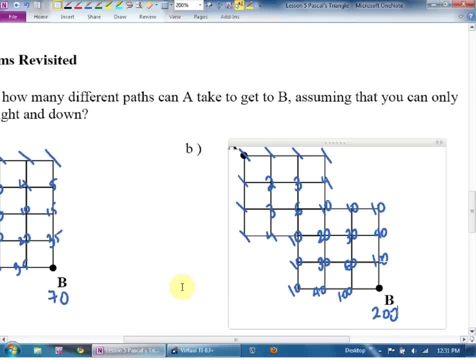 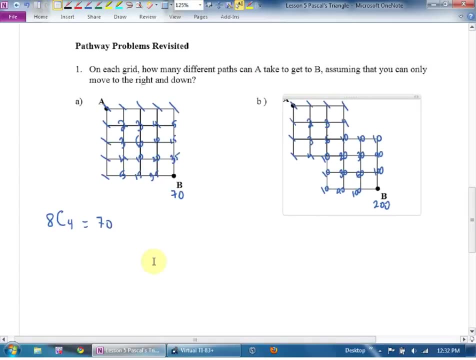 One hundred, No more. See, I mean. What you have to be very careful of is don't make a dumb math mistake, because that will then domino through the rest of your work. There is going to be on the written section of your test. 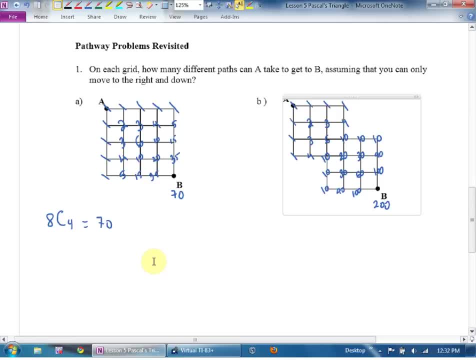 an irregular pathway problem? Because I have to admit that is way high cool on my nerdy list of wow. who knew that Pascal's Triangle could solve pathway problems by adding? By the way, what we're really saying is because these are chooses. 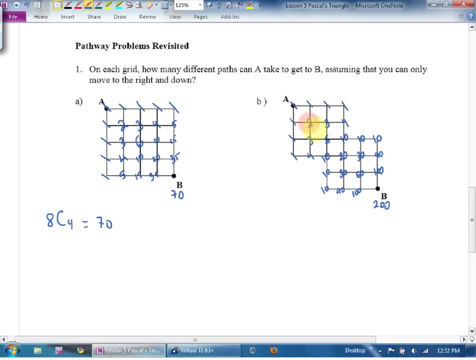 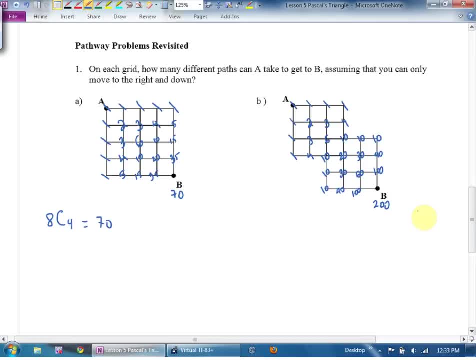 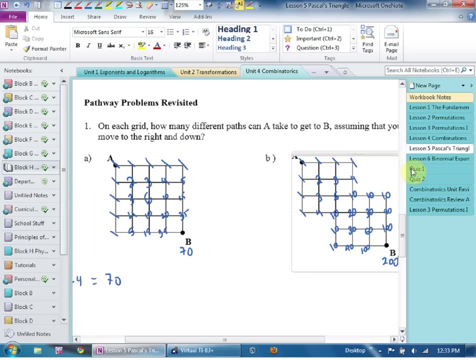 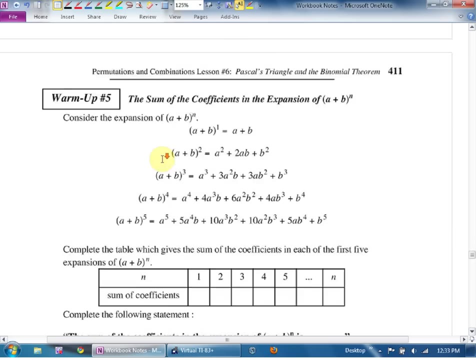 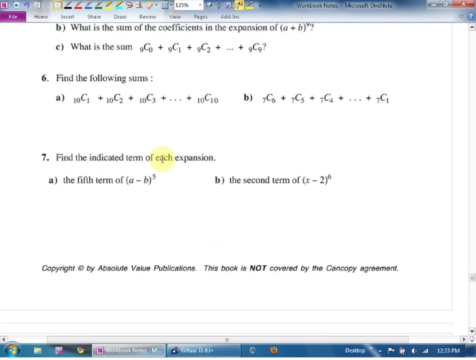 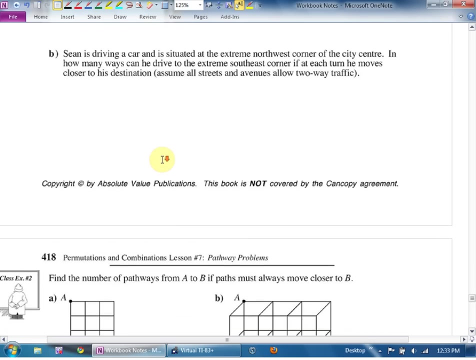 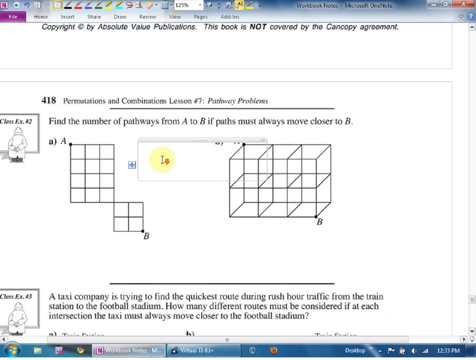 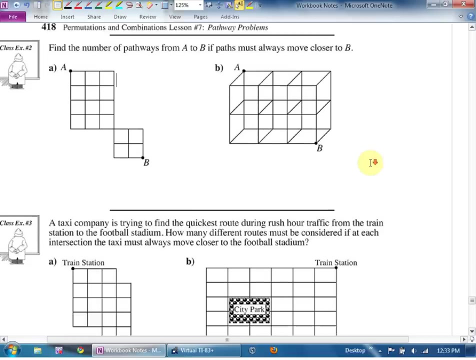 That's why it works. Can you do me a favor, please, and open your workbooks to page Page Page. it's less than seven, So page 418.. 418.. Okay, And on page 418, we have a bunch of little pathway questions. 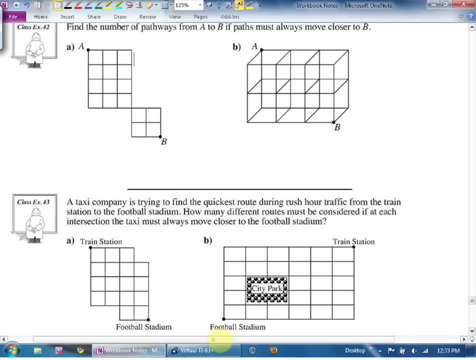 Okay, Page 418, we're there. This here is a regular pathway problem, because, even though there's two different rectangles, can you see there's no overlapping squares. This is an irregular pathway problem, as is this because you have missing or overlapping squares. 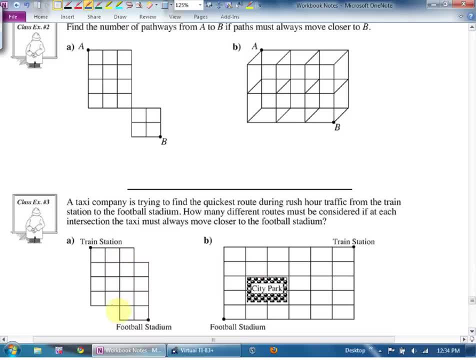 So it's very tough for me to give you a definition, but I'm hoping you can see the difference between that and that This one. we can use a shortcut for Now to do this one. what we're going to do is we're actually going to temporarily in our minds. 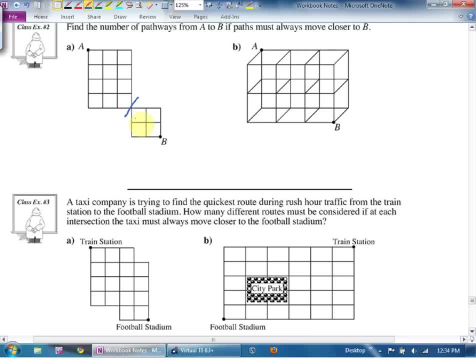 chop it right there. We're going to solve this as two separate rectangles. So this first rectangle it would be right, right, right, down, down, down down. How many letters in this word Seven. So you could either go: 7 factorial over 3 factorial, 4 factorial. 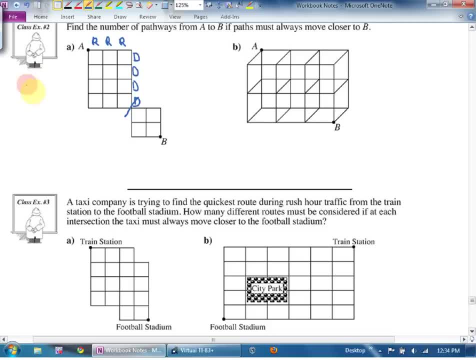 or you could say that just happens to be 7 choose 3,, which is less typing. It's also 7 choose 4, so it doesn't matter whether you went down, down, down, down, down, right, right, right first. 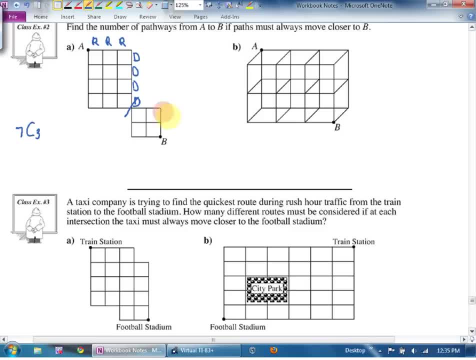 This rectangle- here I'll change colors- would be right, right down down. How many letters in this word? In fact, this one's going to be 4, choose 2.. What's the total? Listen closely, listen closely, listen closely. 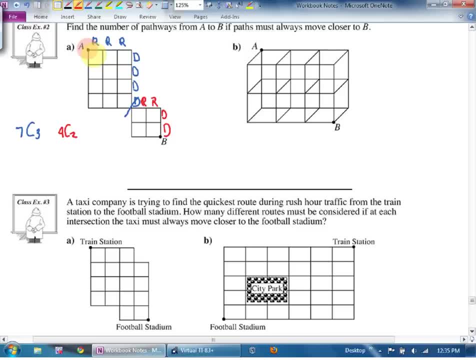 Starting here, I have to go through here and through here. What does and mean Multiply In combinatorics? it means multiply. By the way, you can also solve that one with Pascal's triangle. That's faster Right. 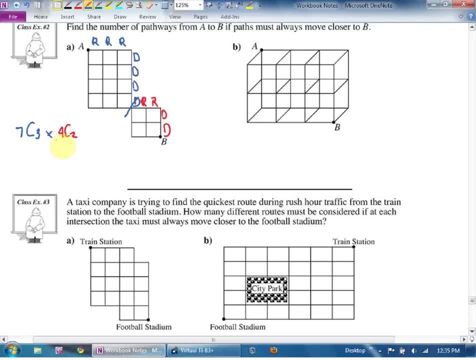 But Pascal would also get you there. What's the answer? 7, choose 3 times 4, choose 2.. How many different pathways are there for that one? How many 210? Is there? I keep hearing 2, and then I'm missing the second number. 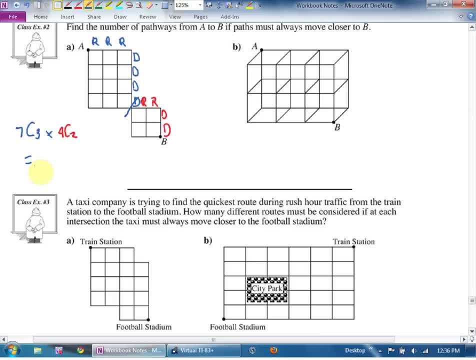 210.. 210.. I thought it was more than 2.. Okay, 210.. Ooh, What about 3D? Do you notice? we're starting at the back of the page and finishing at the front of the page. This one would look like this: 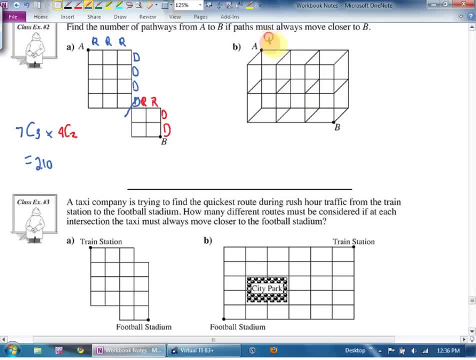 Right right, right Down down. Right right, right Down down, Right right, right Forward. How many letters in this word? grand total: 6 factorial. How many Rs? 3 factorial. How many downs? 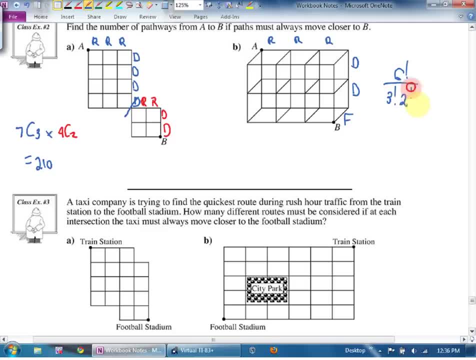 2 factorial. Do those two add to 6? Then I can't use choose as a shortcut. The reason I could use choose as a shortcut here is because 3 plus 4 added to 7, and that was 7. choose 3.. 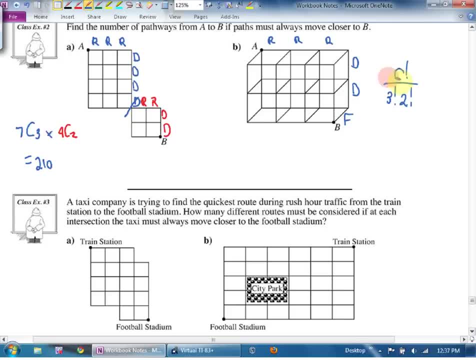 This is not 6, choose 3.. This is 6 factorial over 3 factorial. 2 factorial, Although I would go 12 on the bottom on my calculator. What is 6 factorial divided by 12?? How many pathways? 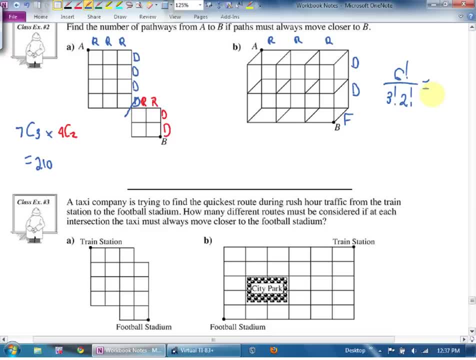 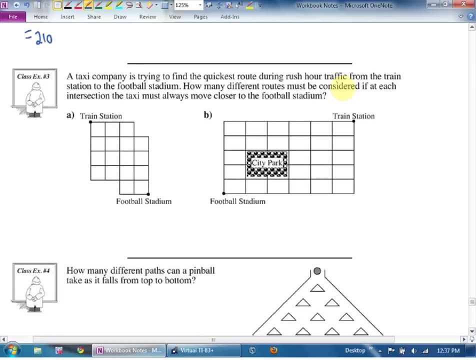 60?. So both of these I was able to use factorial notation because they were regular pathway problems. Ah, the fun ones, the irregular pathway problems. Do you want to try A on your own, or do you want to do it together with me? 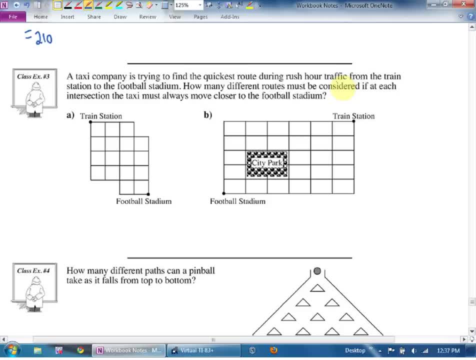 Or do you want me to do it with you, with you not writing anything, and then you try and recreate? Okay, let's do that Ready, So I'll do this with you. If you want to try this solo, just ignore me. 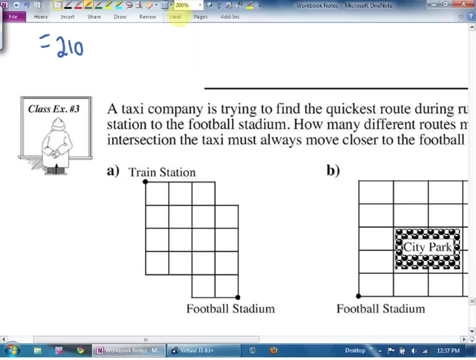 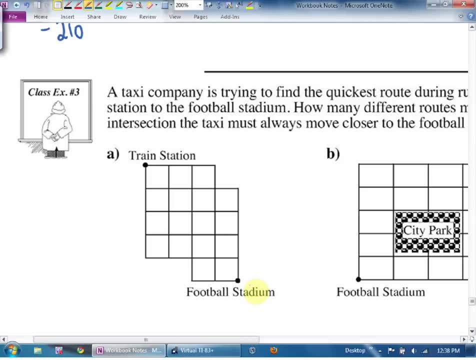 and see if we get to the same spot. Now we're going from the train station to the football stadium. By the way, one nice thing about pathway problems is you get the same answer starting here and going this way, and sometimes one direction is easier than the other. 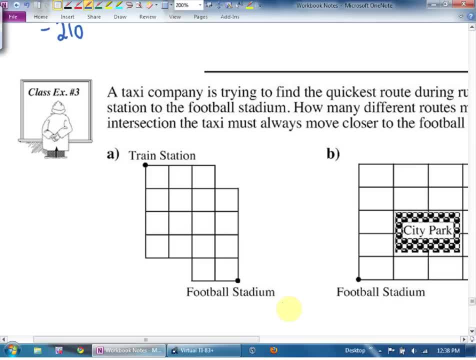 Same answer: 1,, 1,, 1., 1,, 2,, 1., 1,, 3., 3. 3.. 1. 1., 1., 4., 4. 6.. 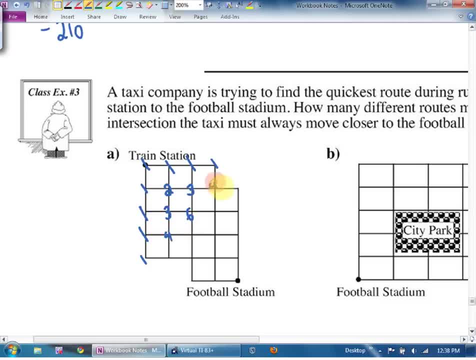 6., 6., 4., 4., 5., 5., 10., 10., 10.. Oh, what number is right here? It's invisible. Right here, Not a 1. What number is right here? 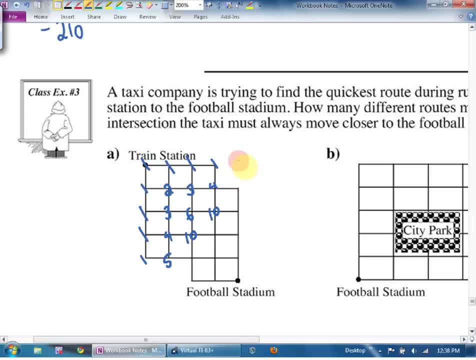 It's invisible. 0.. Right, It's going to be 4 plus. you know what A 4 is going to go there again, because that's the confusing part for most kids, right, Right, 15,, 20,, 14.. 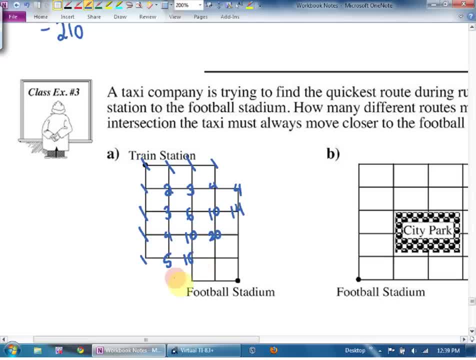 What number is right here, Kim? It's invisible. So the 15 plus 0 is going to give me a 15.. 15 and 20 is going to give me a 35.. 20 and 14 is going to give me a 34.. 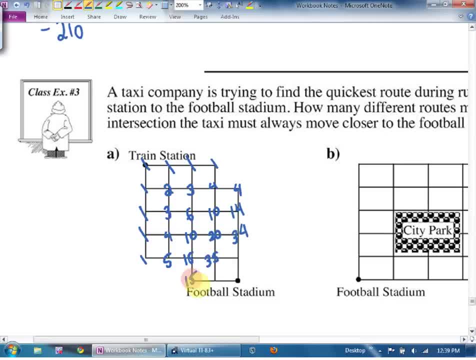 15 and 35 is 50,, 69,, 119.. Now, if you didn't get 119, what you want to do is work your way backwards along the triangle and where you first spot, you see it, sorry, work your way frontwards along the triangle. 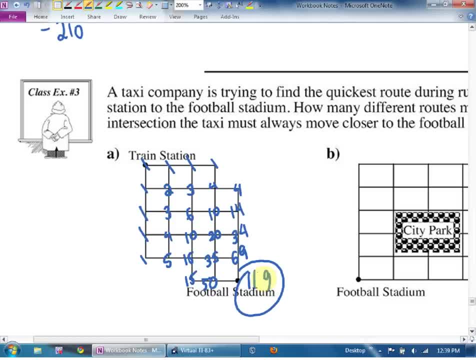 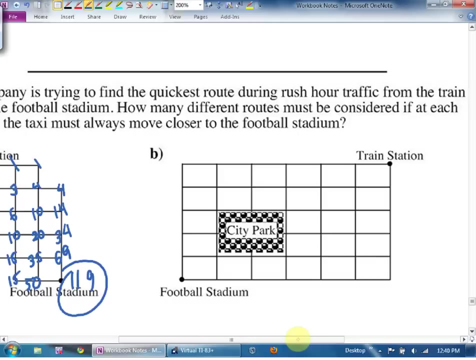 first spot you see a number different from me- is where you make a mistake. Is that okay? We can even nick with this method. cut out squares for a park, like in B. Oh, by the way, did you guys rotate your book 45 degrees? 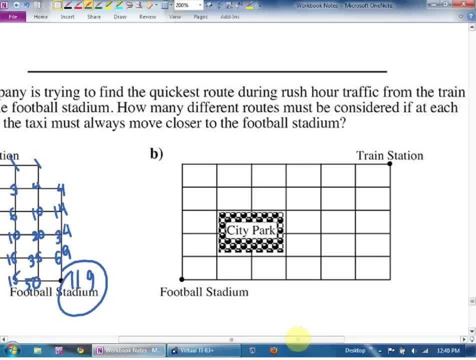 so that the train station was. You think I'm joking. Trust me, I've learned kids make way fewer mistakes because you're adding vertically, which is what you're used to from elementary school. So we're going to start at the train station up here. 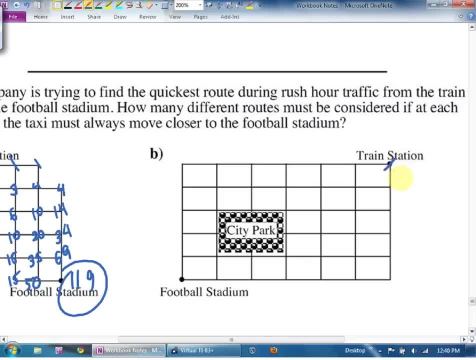 1, 1, 1.. 1, 2, 1.. 1, 3, 3, 1.. 1, 4, 6.. 6, 4, 1.. Now we're getting to the weird stuff. 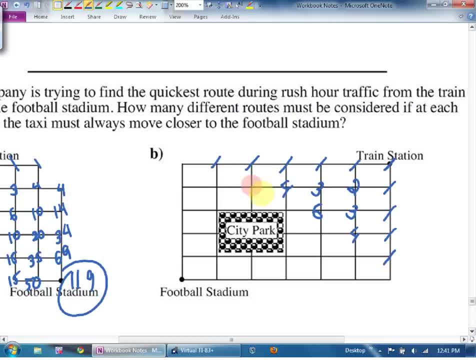 1, 5,, 10.. 10, 5, 1.. 1, 6,, 15,, 20.. 15, 6.. Okay, okay, 1 plus 6, 7.. 6 plus 15, 21.. 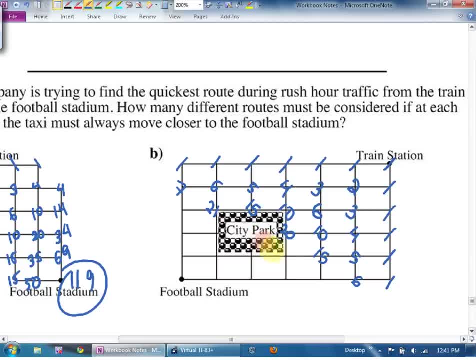 Nothing, nothing, nothing, nothing. 20 plus 15,, 35.. 21. 8. What's going to go right here, Kim? 21 plus nothing. right, There's a zero here. So 21 is just going to drop down like a domino. 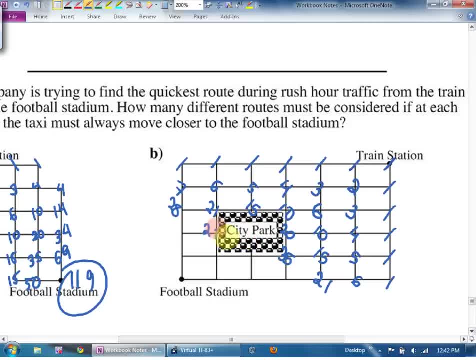 And the 35 is just going to drop down like a domino, And 35 and 21,, 56.. 28 and 21,, 49.. 21 and 35, because both those lines lead here 56.. I think I just did that, didn't I? 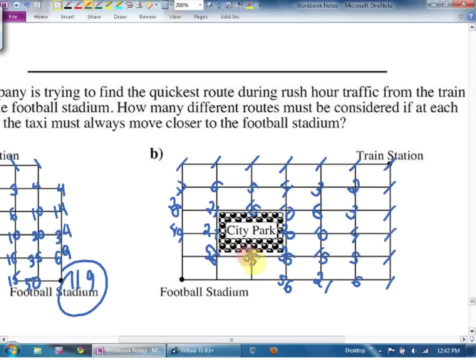 35 and 56,, 86, 91.. 49 and 56, well, 56 and 50 would be 116.. So one less is going to be 105,. Mr Duke, Why'd I go what I can't? because the 49 and the 91 don't join. 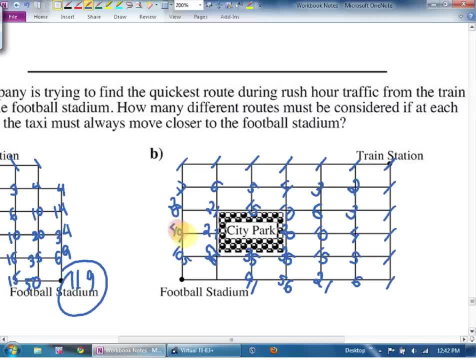 Right, I'm always just going to the two right above me diagonally. It's going to be the 56 and the 91.. 56 and 91, 91 and 50 is going to be 141 plus 147.. Final answer: 105 and 147, 247. 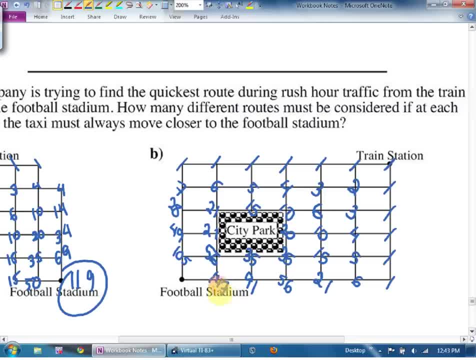 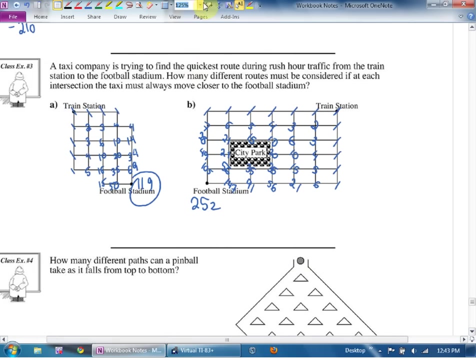 Is the final answer 252?? Is that resultados? I'm going to say performance ratio, Disability, progress, Posings, test results- I'm going to say percentage, Then cuts and totals. Is there something another person is going to do? It's positive or negative? 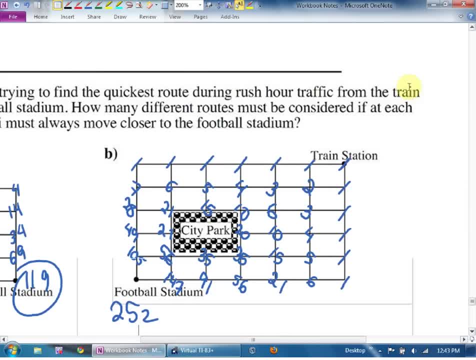 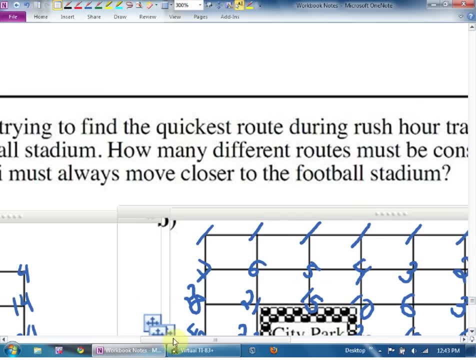 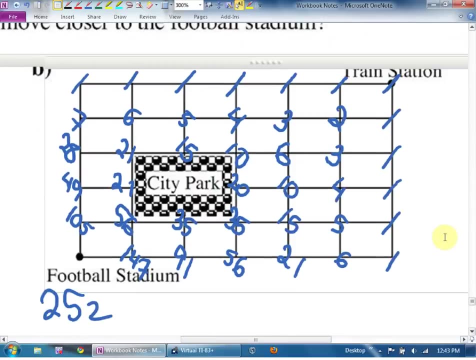 No, I was going to say I don't. I'm going to say SELECT. Oh, SELO, I can get a little bigger if you want me to. still You sure? Uh-huh, There's always an empty spot next to Rio if you need to. 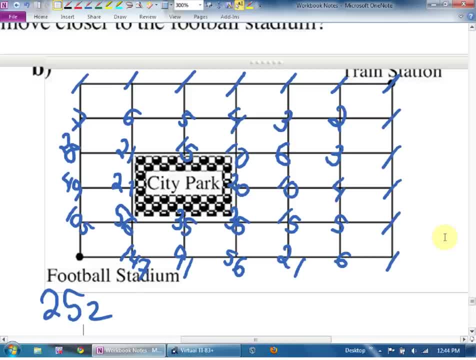 By the way, these ones- those of you that tend to slough on the homework- these ones need practice because they seem easy, But you're going to find little weird curveballs along the way and you'll figure them out once you hit them. 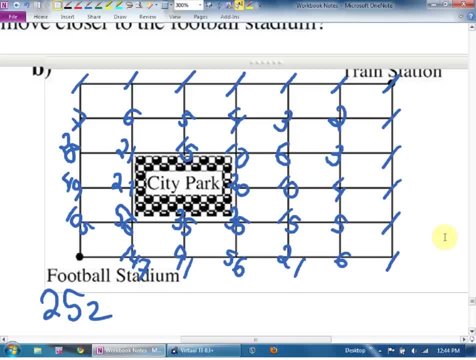 but you don't want to be figuring them out for the first time on a quiz or a test. In other words, I'm kind of saying for those of you that never do the homework tonight: Brent, can I make it smaller? Brent? 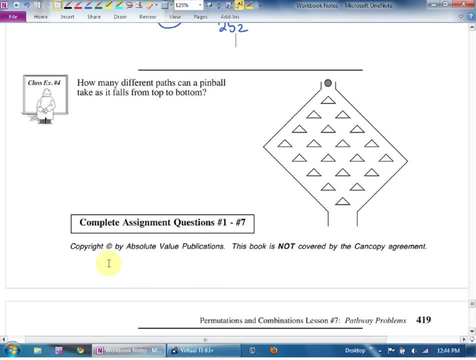 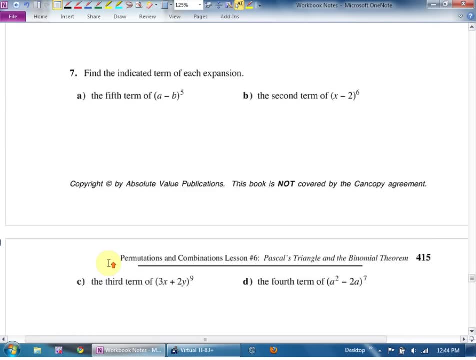 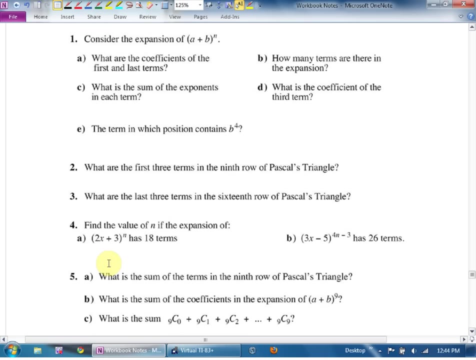 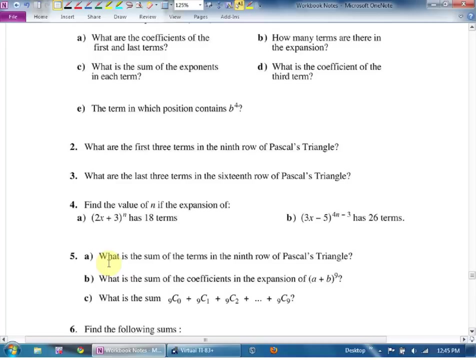 Skip example four. What's your homework? First of all, turn back one lesson, please, to lesson six, To page 414.. So this is some Pascal's Triangle questions, And all I'm going to assign right now is two and three from this unit, from this lesson. 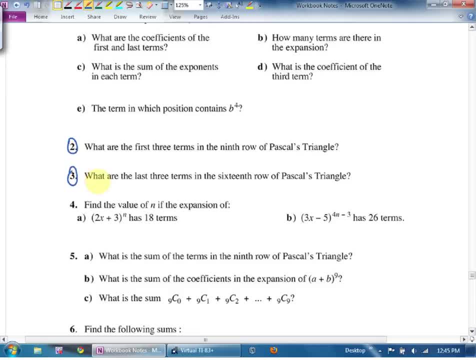 So find the first three terms of the ninth row. Ninth row is going to be- I think it's going to be- eight choose zero, eight choose one and eight choose two. What are the last three terms in the 16th row? 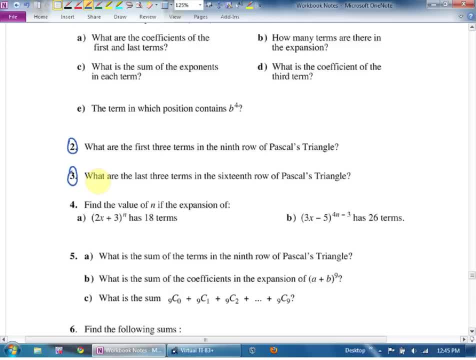 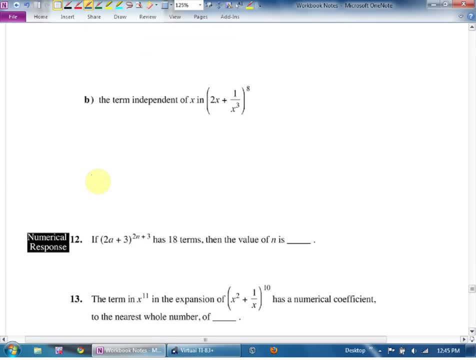 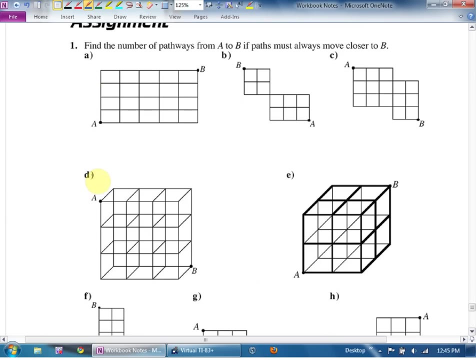 Oh, you think. Think about those. Then turn ahead one lesson, please, to page 419.. One A, that's a regular one. You can use factorial shortcuts. One B, that's two regular ones. Solve them each individually using factorials. 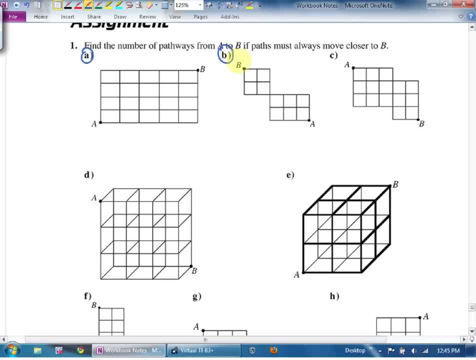 You can use factorial shortcuts and then multiply your answers together, because you've got to go through one and the other. Two C, that is an irregular one. Pascal's Triangle: One C, sorry, one C. One C that's an irregular one. so Pascal's Triangle. 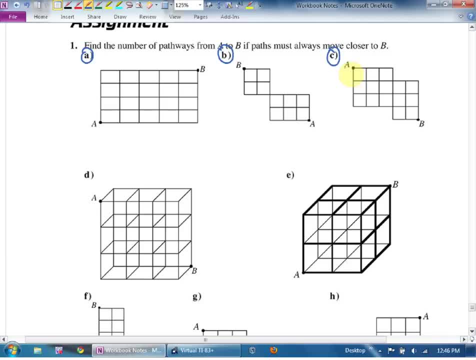 I'll give you one 3D one Now. I've done the three-dimensional ones with you. They've never showed up on the provincial, but I don't know why, because I think they're nerdily cool, So I've covered it, just in case. 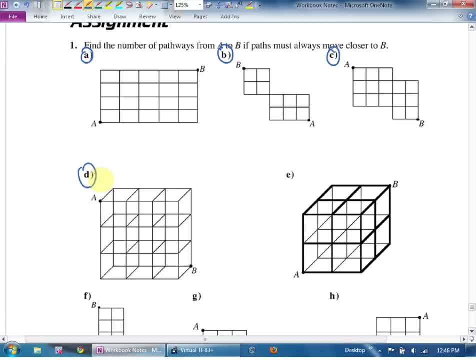 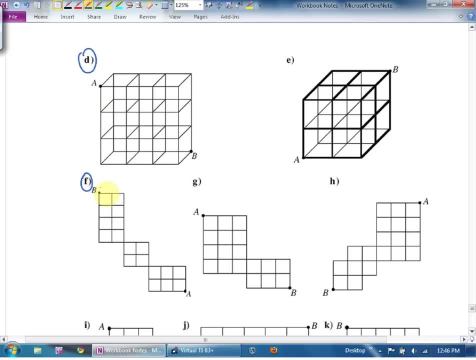 I'm going to skip E. F is good. Now do any. F is made up of three big rectangles. See them. Do they overlap at all? So you can do each one separately. multiply, multiply, multiply. You can do this one and this one and this one using factorial notations. 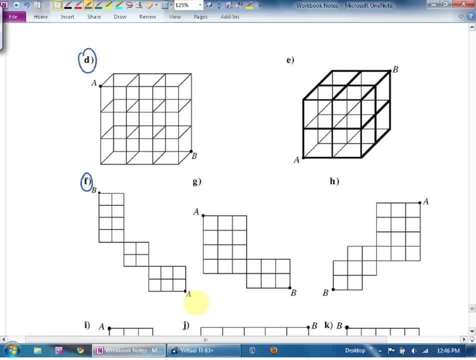 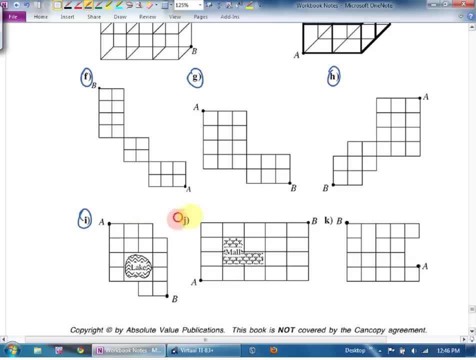 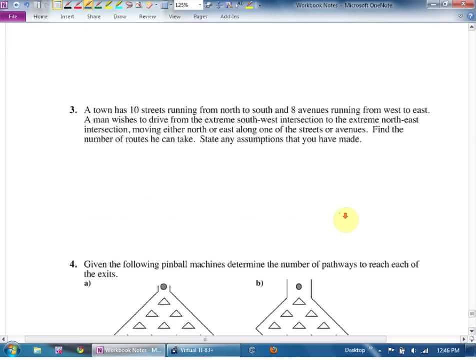 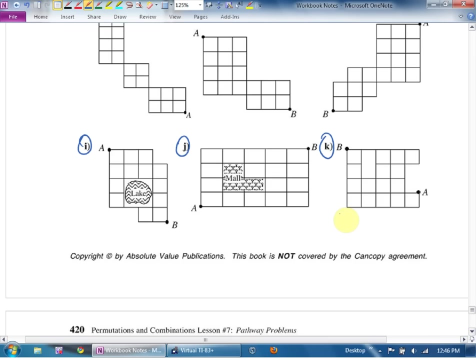 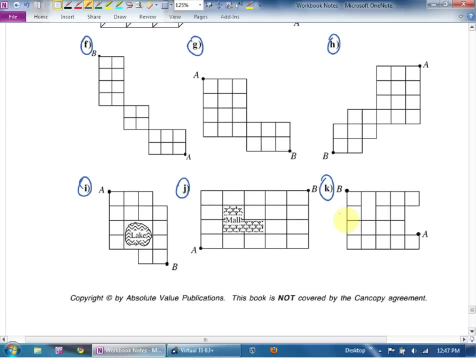 But then let's do the irregular ones. G is good, H is good, I, J and K Okay. Pathway problems and Pascal's grade 3 math solves grade 12 questions. You also have the take-home quiz, Thank you. 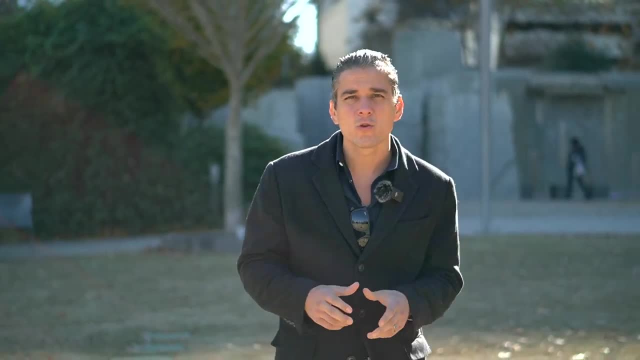 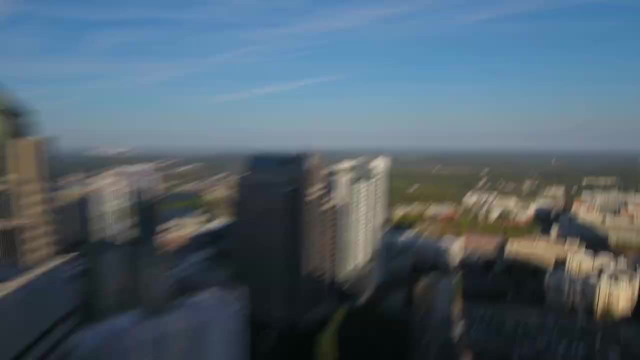 So you're thinking about moving to the Carolinas, but is it North Carolina or South Carolina? Which one should you choose? Which one's better? Well, there's a lot of pros and cons to both North Carolina and South Carolina, and that's exactly what we're going to discuss on today's video.